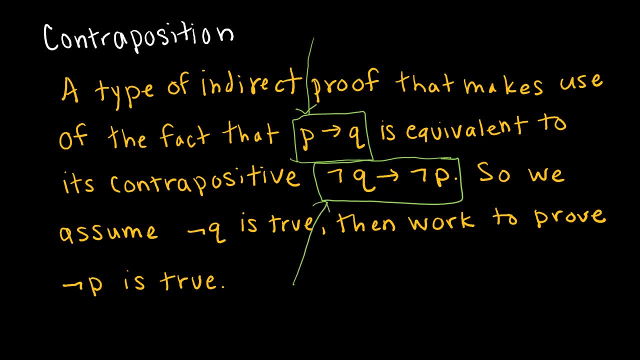 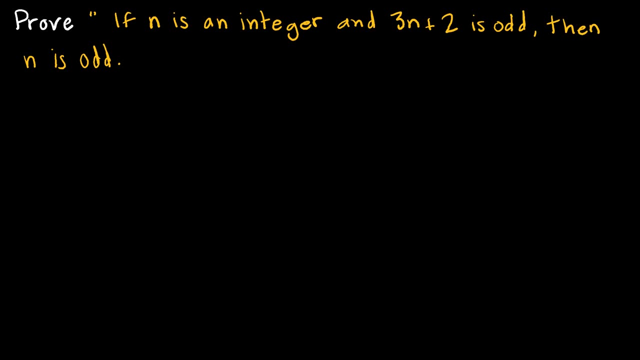 contraposition proof, we're going to assume not Q and we're going to prove not P is true, therefore by contraposition proving that if P, then Q is also true. So let's take a look at our indirect proof and again, in our indirect proof of contraposition we're 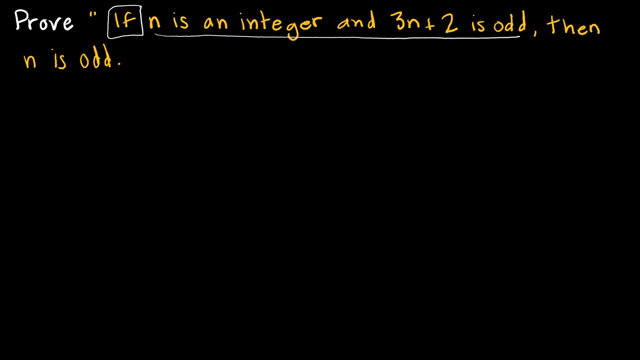 saying: if P, then Q is our implication. we're going to show: not Q implies not P. so here's P and here's Q. and now I'm going to a start by assuming not Q. and if I can show that this relationship is true, it will show that if P, then Q is. 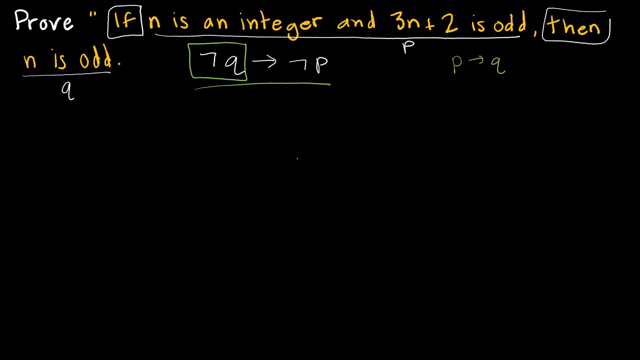 true, which is of course what I'm trying to get to. so let's get started. I'm going to assume N is not odd, so I'm assuming not Q. so not odd is the same as even. so I'm going to assume N is even so N can be represented as 2k. 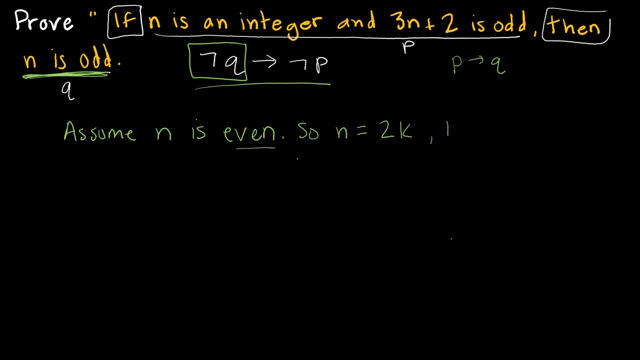 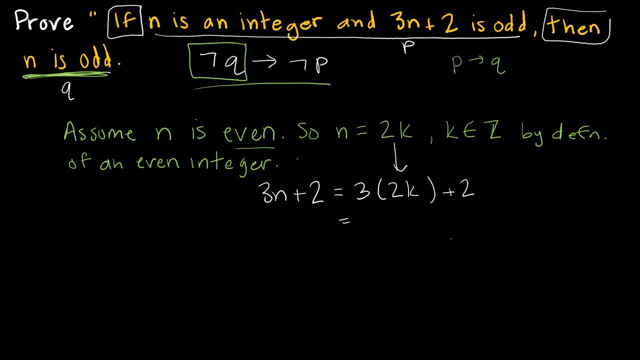 3n plus 2, which is 3- whoops, not 2, 3 times 2k, by 3n plus 2, which is 3- whoops, not 2, 3 times 2k. by substitution plus 2, which is 6 K plus 2. 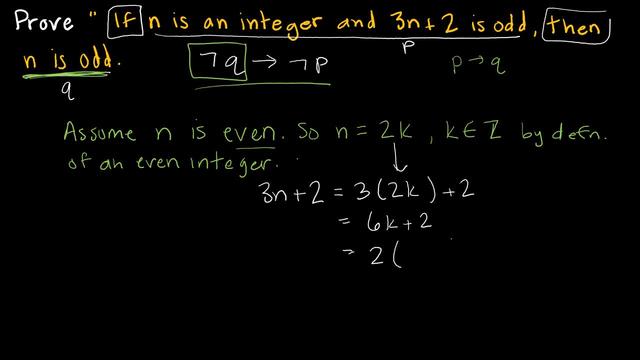 substitution plus 2, which is 6 K plus 2. substitution plus 2, which is 6 K plus 2, which is 2 times some quantity, and that which is 2 times some quantity and that which is 2 times some quantity and that quantity is 3 K plus 1, or just as I did. 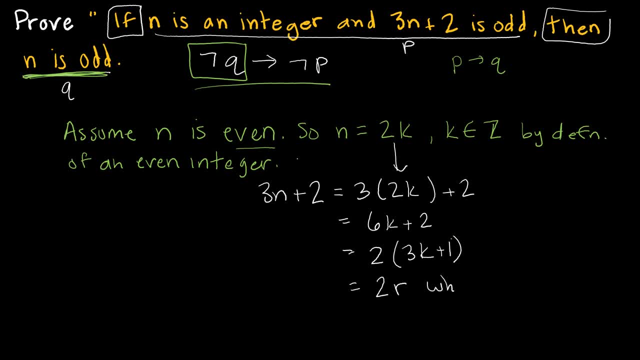 quantity is 3 K plus 1, or, just as I did, quantity is 3 K plus 1. or, just as I did in the last video, I can say 2 R, and in the last video I can say 2 R, and in the last video I can say 2 R. and where R is equal to 3 K plus 1 and R is 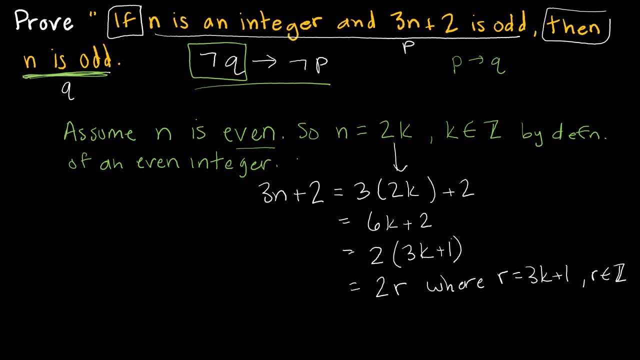 where R is equal to 3 K plus 1 and R is where R is equal to 3 K plus 1 and R is an integer. so what have I just shown? I, an integer. so what have I just shown? I an integer. so what have I just shown? I have shown that not Q implies not P. 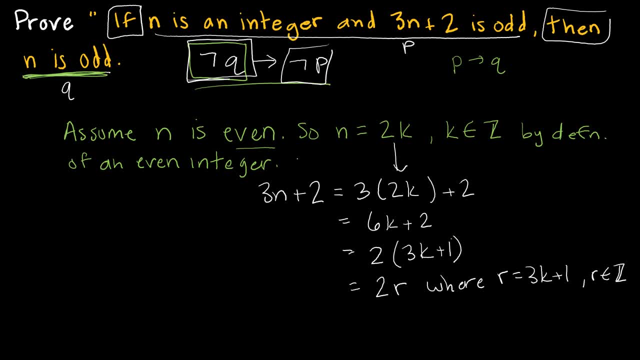 have shown that not Q implies not P. have shown that not Q implies not P. because P says 3 n plus 2 is odd and I because P says 3 n plus 2 is odd and I because P says 3 n plus 2 is odd and I have just shown here that 3 n plus 2 is. 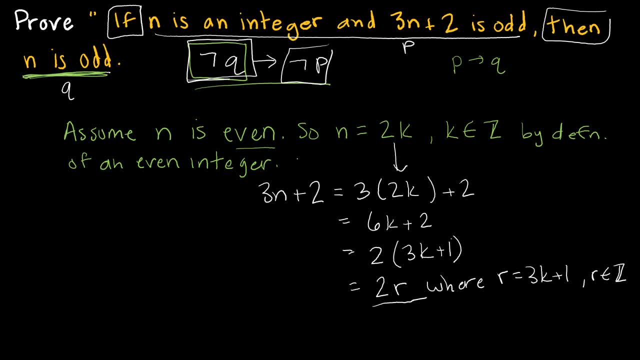 have just shown here that 3 n plus 2 is, have just shown here that 3 n plus 2 is, in fact, even by definition of an, even in fact, even by definition of an, even in fact, even by definition of an even number. so I'm going to say, I'm going, 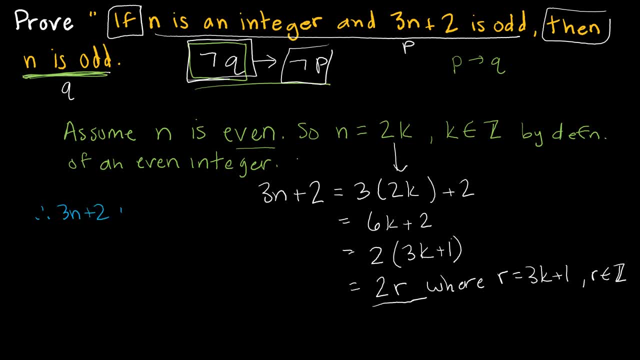 so I'm going to say I'm going, so I'm going. therefore, 3 n plus 2 is, even since not Q implies not P, is true. therefore, 3 n plus 2 is even since not Q implies not P is true. therefore, 3 n plus 2 is, even since not Q implies not P is true. then, if P, then Q is true. 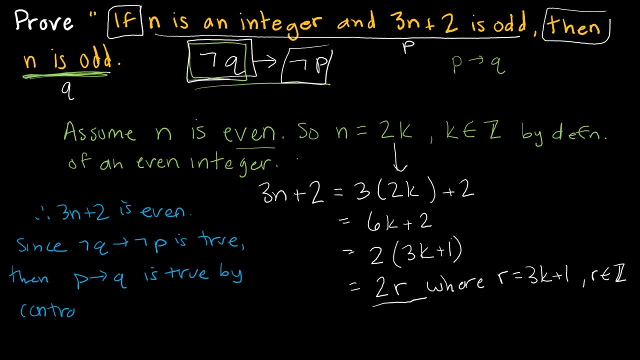 then if P, then Q is true. then if P, then Q is true. by contraposition, and again by contraposition, and again by contraposition, and again QED or your box or your triangle, or QED or your box or your triangle, or QED or your box or your triangle, or however you're ending your proofs. 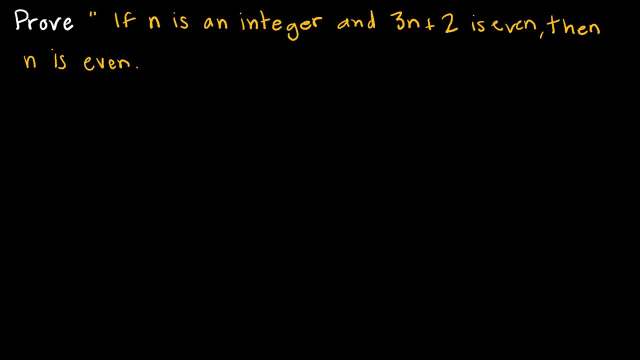 however, you're ending your proofs. however, you're ending your proofs. here's another one for you to try, and here's another one for you to try, and here's another one for you to try, and I'd really like you to try this one on. I'd really like you to try this one on. 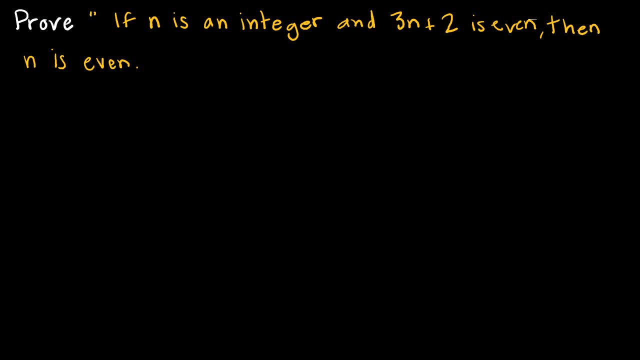 I'd really like you to try this one on your own, because it's exactly the same, your own. because it's exactly the same, your own, because it's exactly the same proof. we just did, except I've replaced proof. we just did, except I've replaced proof. we just did, except I've replaced these with. even so, if you would press, these with. even so, if you would press these with. even so, if you would press pause, try this question on your own when pause. try this question on your own when pause. try this question on your own when you're ready. press play to see how you. you're ready. press play to see how you. 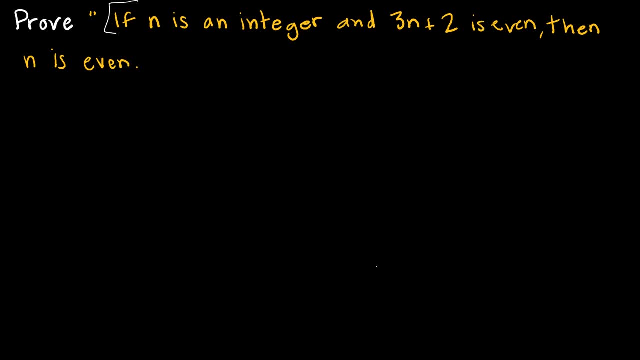 you're ready. press play to see how you did so again. I'm still working with the. did so again. I'm still working with the. did so again. I'm still working with the same. if P, then Q, so here's P, here's Q. same. if P, then Q, so here's P, here's Q. 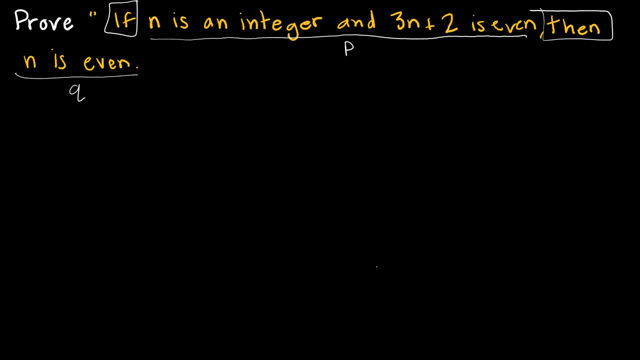 same. if P, then Q. so here's P, here's Q, and in a proof by contraposition I'm, and in a proof by contraposition I'm, and in a proof by contraposition I'm going to assume not Q, so I'm going to. 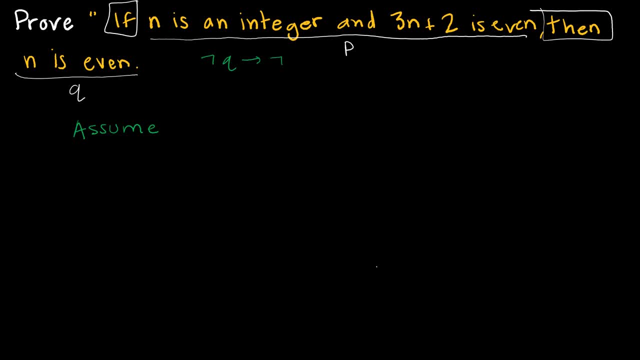 going to assume not Q. so I'm going to going to assume not Q. so I'm going to assume not Q. show that that implies not. assume not Q. show that that implies not. assume not Q. show that that implies not P. that's going to tell me: if P, then Q is. 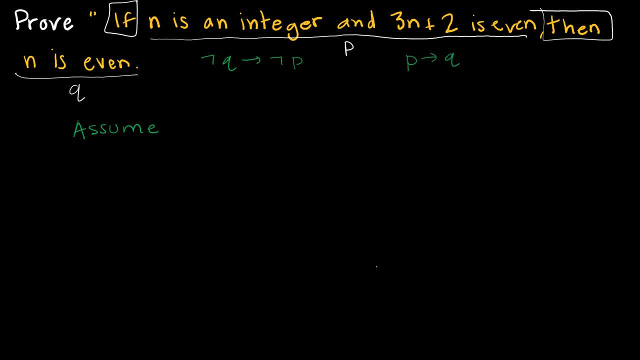 P. that's going to tell me. if P, then Q is P. that's going to tell me. if P, then Q is also true. so I'm going to assume n is also true. so I'm going to assume n is also true. so I'm going to assume n is not even, or assume n is odd. and if n is, 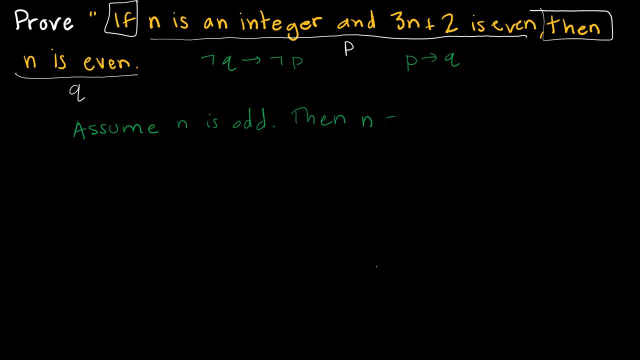 not even or assume n is odd. and if n is not even or assume n is odd. and if n is odd, then n can be written as 2 K plus 1 odd, then n can be written as 2 K plus 1 odd. then n can be written as 2 K plus 1 for some integer K. so if that's the case, 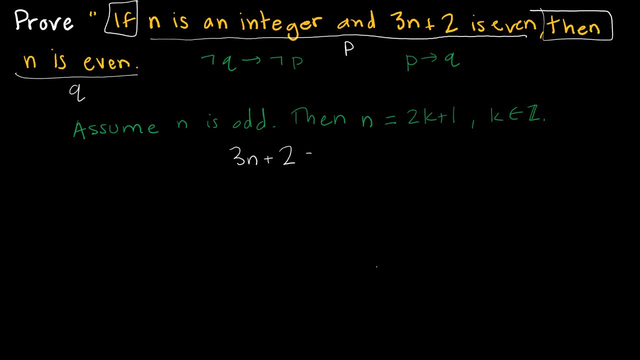 for some integer K. so if that's the case for some integer K. so if that's the case, then I can take 3 n plus 2 and replace. then I can take 3 n plus 2 and replace. then I can take 3 n plus 2 and replace n with 2 K plus 1, whoops, and then I can. 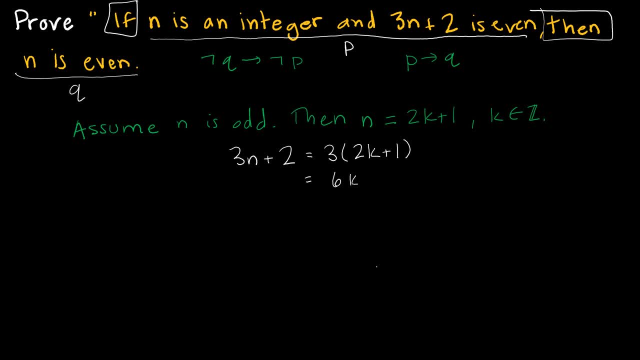 n with 2 K plus 1 whoops, and then I can n with 2 K plus 1 whoops, and then I can rewrite that as 6 K- oops, I forgot, rewrite that as 6 K. oops, I forgot, rewrite that as 6 K. oops, I forgot something. this is plus 2, so this is now. 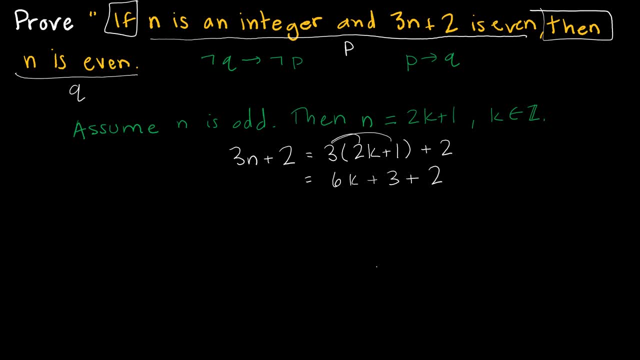 something. this is plus 2. so this is now something. this is plus 2. so this is now 6 K plus 3 plus 2, and keep in mind where 6 K plus 3 plus 2, and keep in mind where 6 K plus 3 plus 2, and keep in mind where we're trying to head is we're trying to. 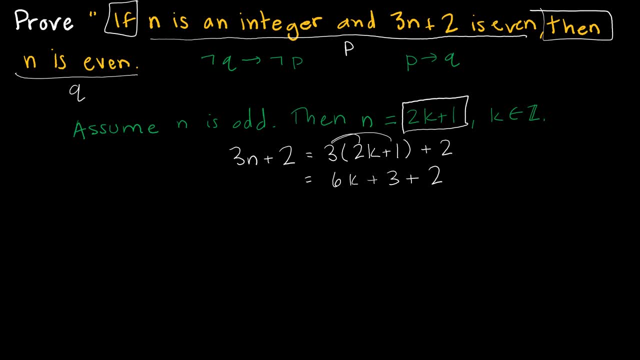 we're trying to head is we're trying to. we're trying to head is we're trying to keep things either in this format or in. keep things either in this format or in. keep things either in this format or in the n equals 2 K format. so I'm going to. 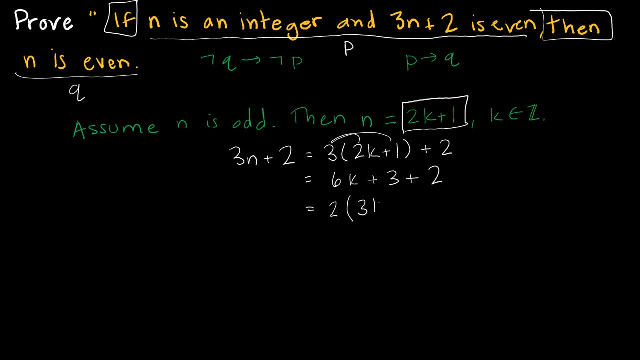 the n equals 2 K format. so I'm going to the n equals 2 K format. so I'm going to rewrite this as 2 times and that would rewrite this as 2 times, and that would rewrite this as 2 times and that would be 3 K, and then I have a total of 5 here. be 3 K, and then I have a total of 5 here. be 3 K, and then I have a total of 5 here. but notice, I've got a 2 here, so I'm. but notice, I've got a 2 here, so I'm. 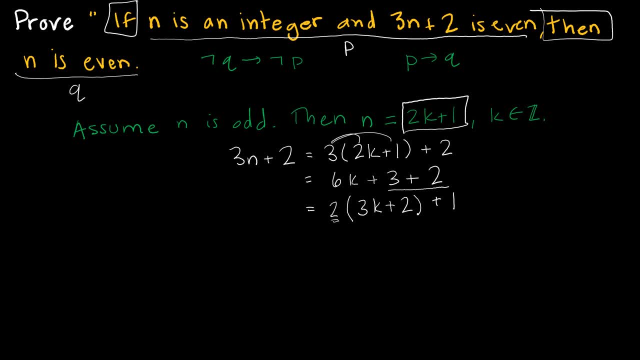 but notice, I've got a 2 here, so I'm going to say plus 2, which gives me 4, going to say plus 2, which gives me 4, going to say plus 2, which gives me 4, with one left over. and of course I did. 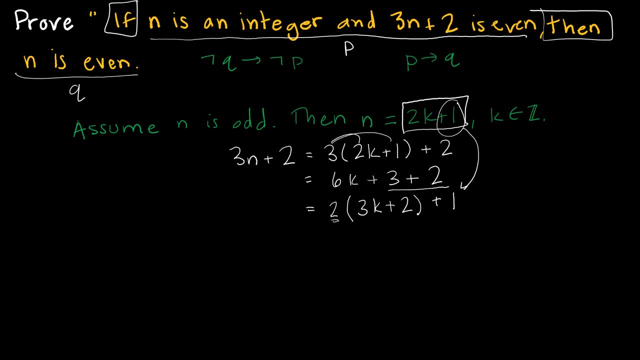 with one left over. and of course I did with one left over, and of course I did that because that gives me that one, that, because that gives me that one, that, because that gives me that one left over on the outside, just as before I left over on the outside, just as before I.